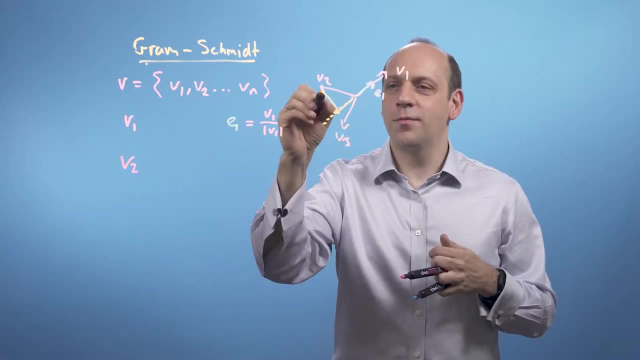 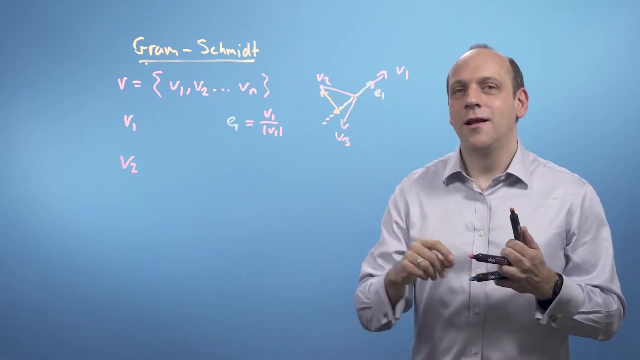 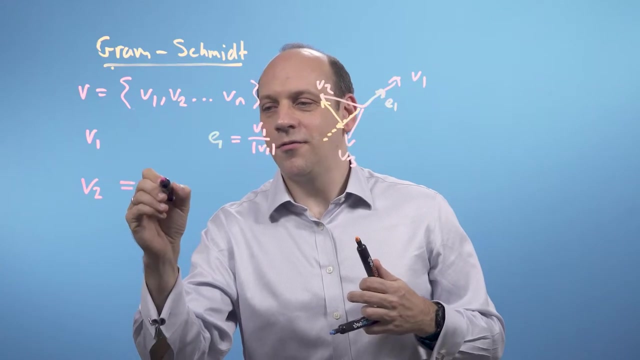 the direction of e1, like that, plus a component that's perpendicular to e1., And but the component that's in the direction of e1, I can find by taking the vector projection of v2 onto e1. So I can say v2 is equal to the vector projection of v2 onto e1, dotted together. 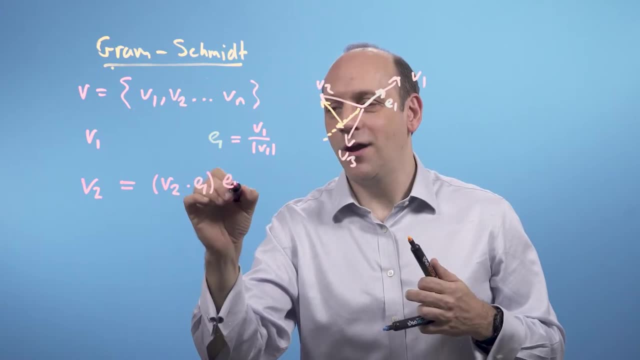 And if I want to get that actually as a vector, I'll have to take e1, which is of unit length. I'd have to divide by the length of e1, but the length of e1 is 1, so forget it. 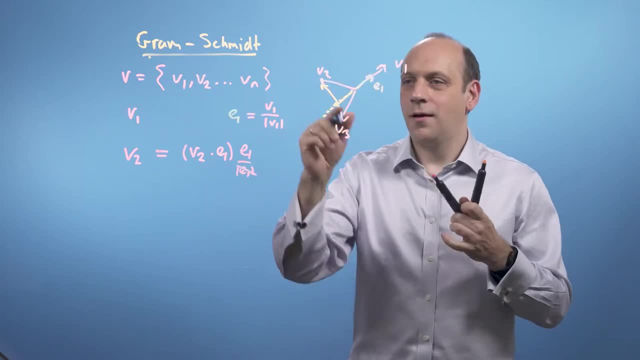 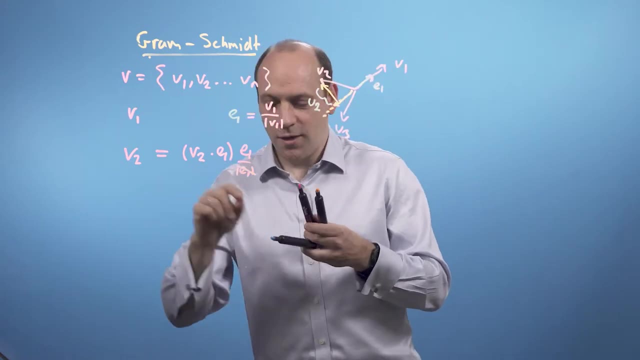 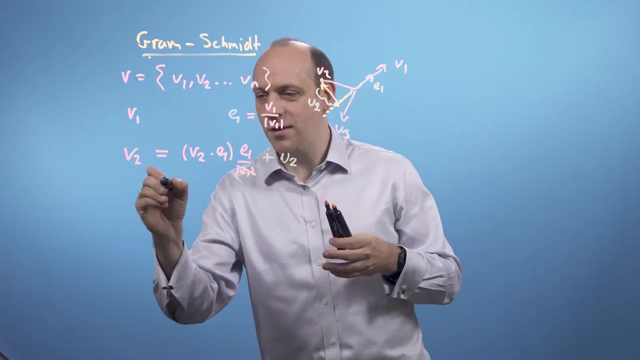 And if I take that off of v2, then I'll have this guy and let's call him u2.. So I can then say that u2, so plus u2, so I can then rearrange this and say that u2.. 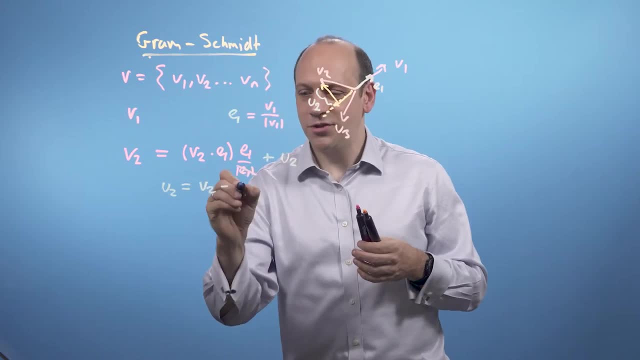 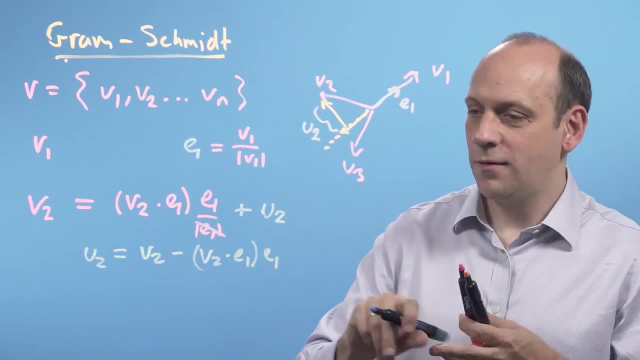 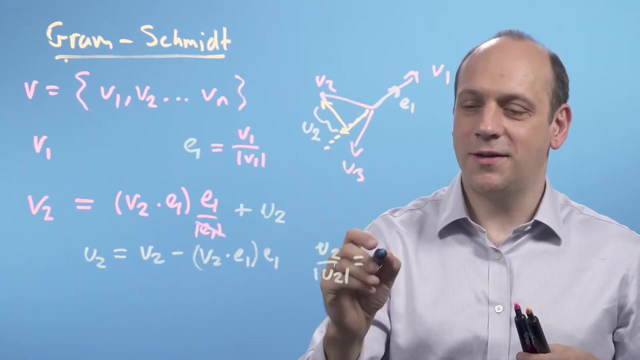 Is equal to v2, minus this projection, v2.e1 times e1.. And if I normalize u2, if I take u2 divided by its length, then I'll have a unit vector which is going to be normal to v1. 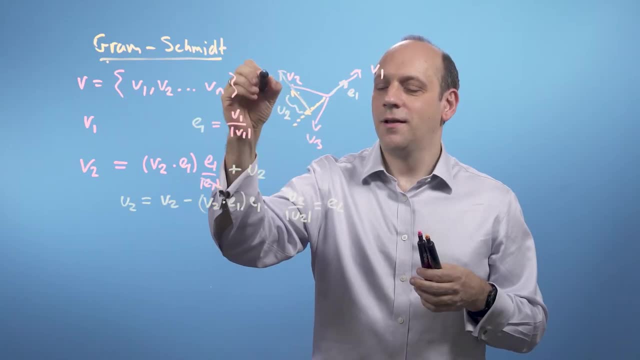 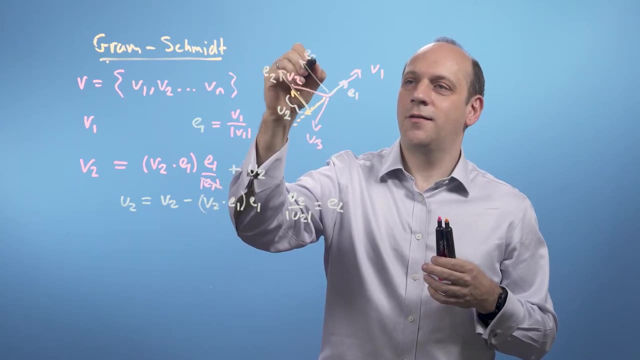 So if I take a normalized version of that, let's say it's that that will be e2, and that will be at 90 degrees to e1.. Okay, So it'll actually be there e2, once I've moved it over. 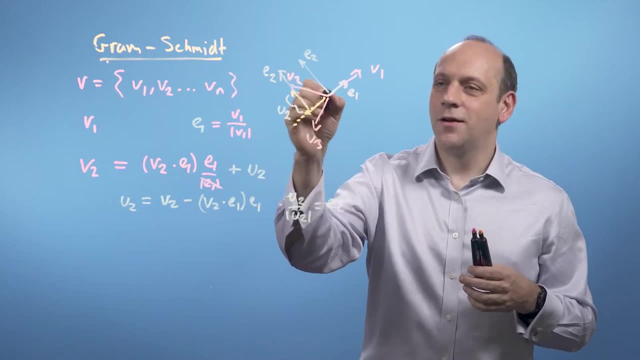 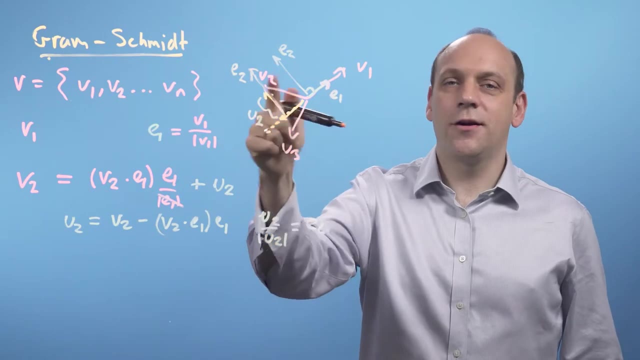 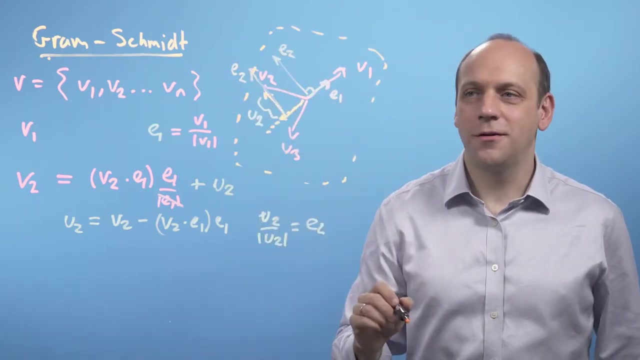 And that will be another unit length vector, normal to e1.. So that's the first part of taking an orthonormal basis. Now my third vector- v3, isn't a linear combination of v1 and v2. So v3 isn't in the plane defined by v1 and v2.. 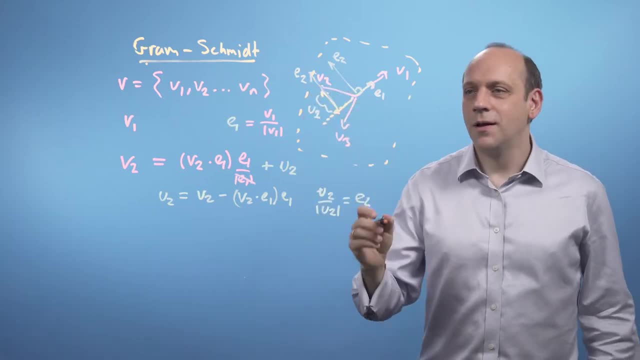 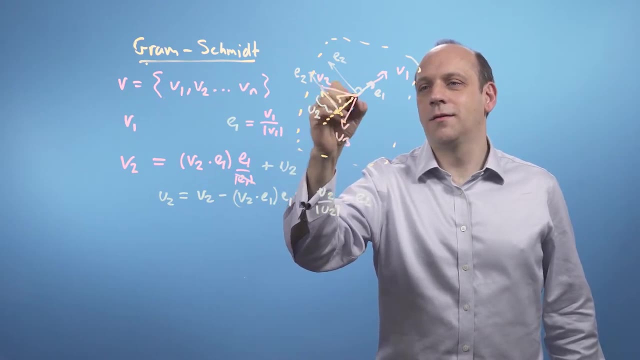 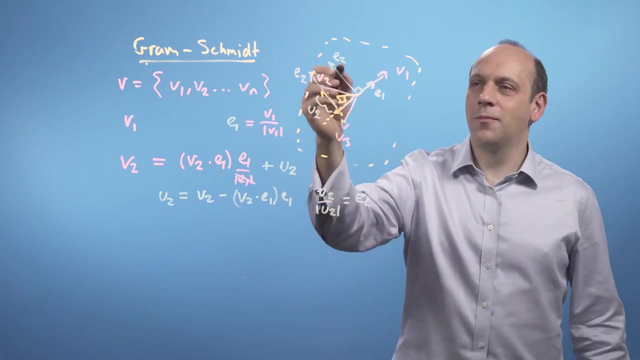 So it's not in the plane of e1 and e2 either. So I can project v3 down- Let's say something like that- onto the plane of e2 and e1, and our projection will be some vector in the plane composed of e2s and e1s.